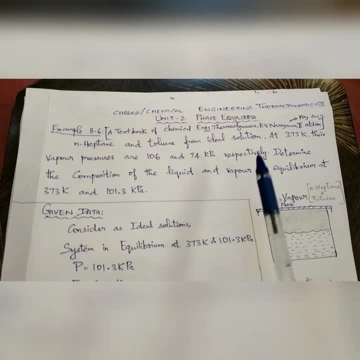 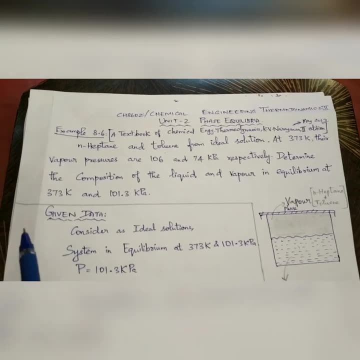 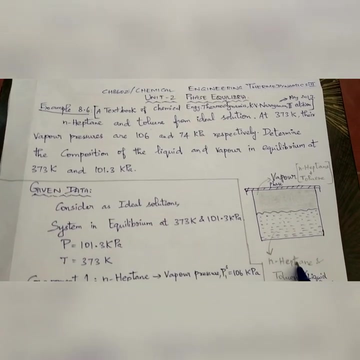 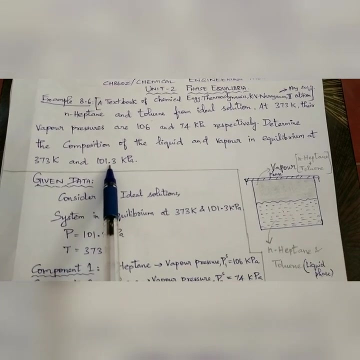 I had taken a problem in K B Narayanan a textbook of Chemical Engineering, Thermodynamics book, example 8.6, the phase equilibrium. I am taking a system which, having n-heptane and toluene in liquid phase and the equilibrium condition at 373 and 101.3 kilopascal pressure, which is maintained, 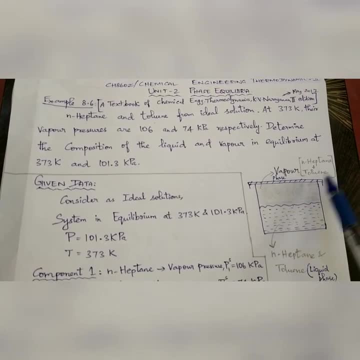 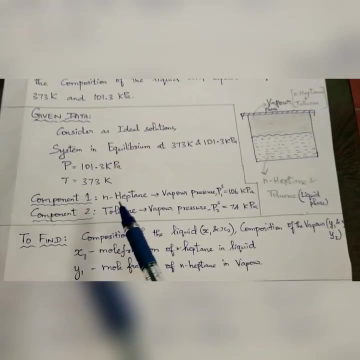 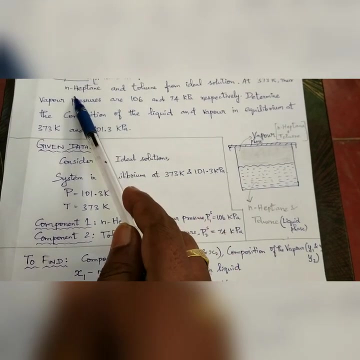 It will form vapor. The vapor phase Also consists of n-heptane and toluene. So from this problem we are going to find mole fraction or composition of the liquid and vapor in equilibrium condition of n-heptane and toluene. 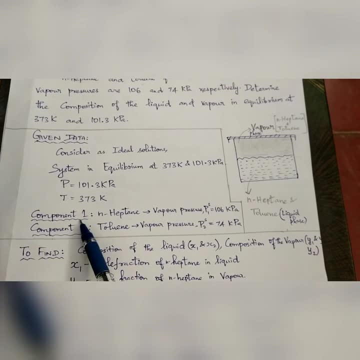 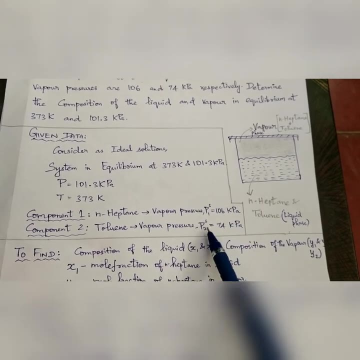 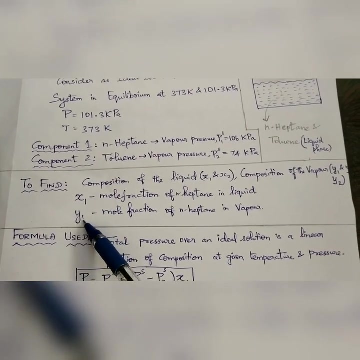 So I have taken n-heptane as component 1 and toluene as component 2.. The respective vapor pressures are 106 kilopascal and respective pressure 74 kilopascal. for toluene, I am going to find x1 as well as y1.. 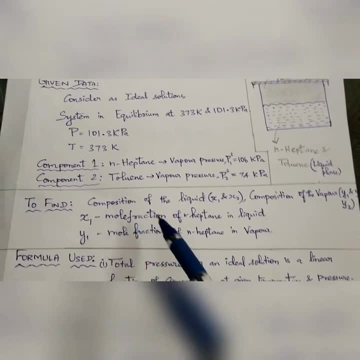 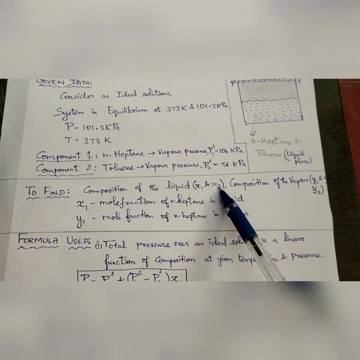 What does it mean by x1 and y1?? x1 is nothing but mole fraction or composition of n-heptane in liquid phase. Similarly x2.. What does it mean by x2? Mole fraction of toluene in liquid phase. 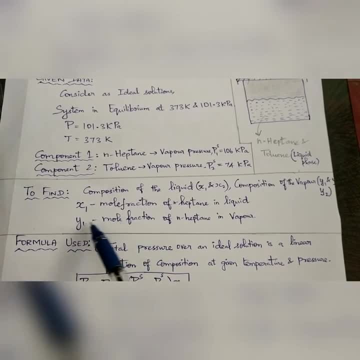 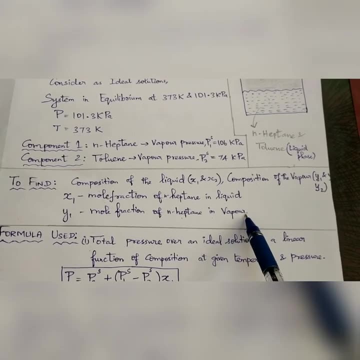 Like that composition of vapor y1. It is considered as y1. And mole fraction y1 is taken as mole fraction of n-heptane In vapor phase And y2 is nothing but mole fraction or composition of toluene in vapor state. 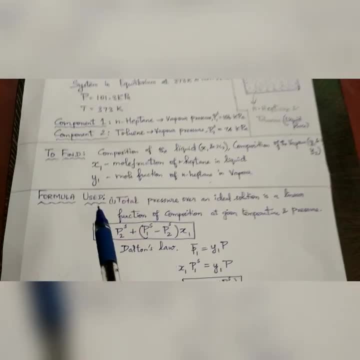 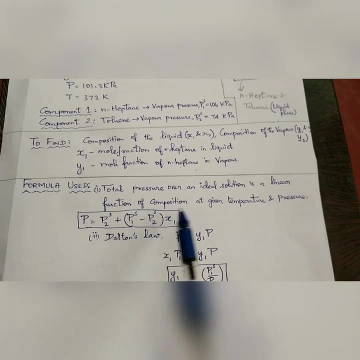 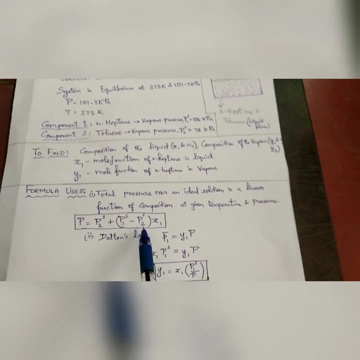 So formula used for this problem is total pressure over. an ideal solution is a linear function of composition at given temperature and pressure. Capital P equal to P2s plus P1, minus P2 into x1.. Second formula is, according to Dalton's law: 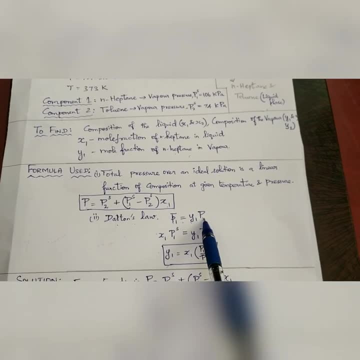 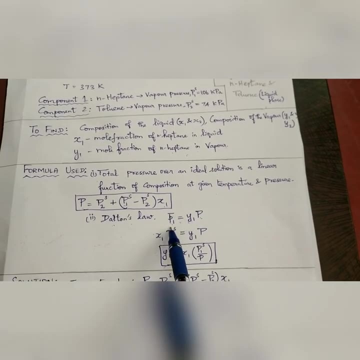 We know that P1 bar is equal to y1 into P. P is nothing but total pressure, Y1 is nothing but mole fraction of n-heptane in vapor state And P1 bar is nothing but partial pressure with respect to the liquid state. 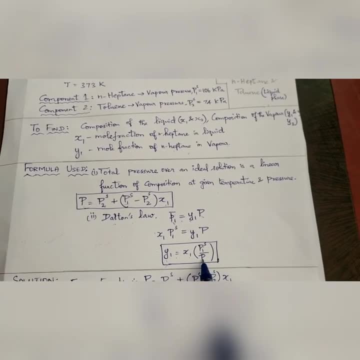 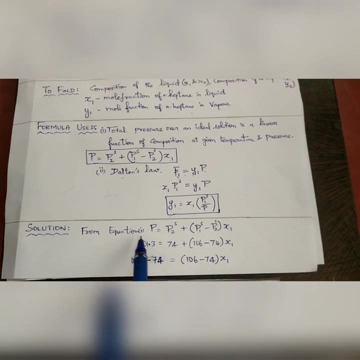 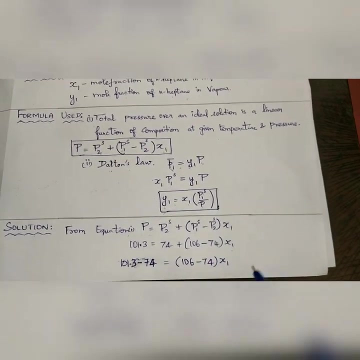 So y1 equal to x1 into P1 by capital P. Finally, we have time. Solution From equation 1, we substitute the respective pressures in the equation 1.. We get x1.. We are going to find x1..